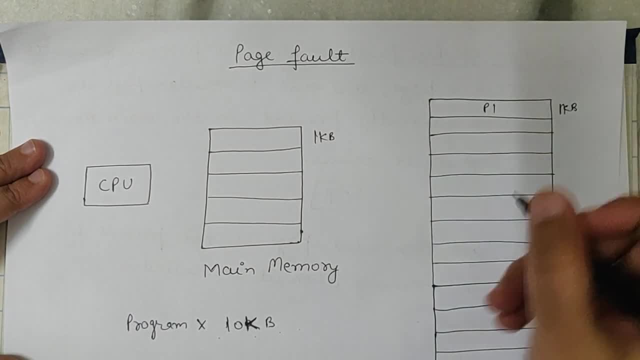 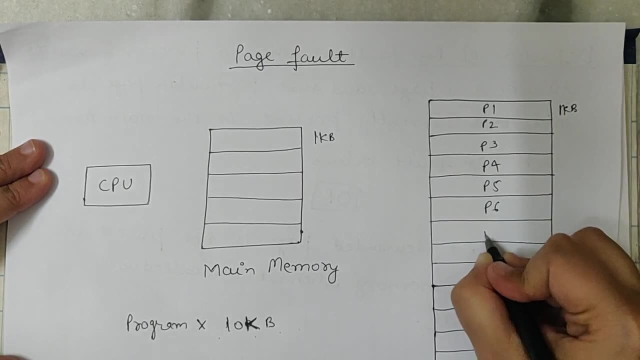 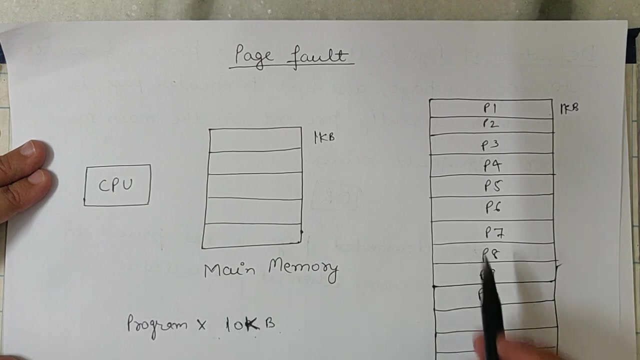 Okay, so let's say this is P1, page P1, size 1 KB, P2, P3, P4, P5, P6, P7, P8, P9 and P10.. So this program X, which is of size 10 KB, occupies this 10 KB space. Okay, P1, P2, P3,. 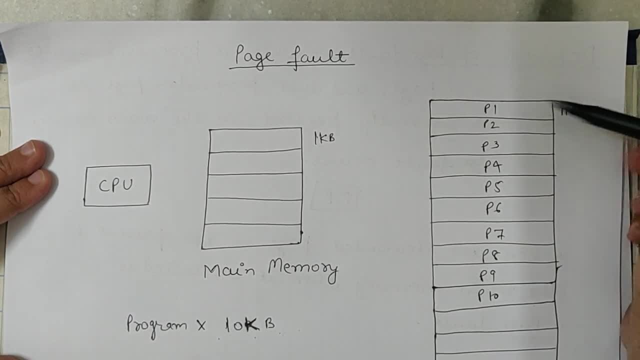 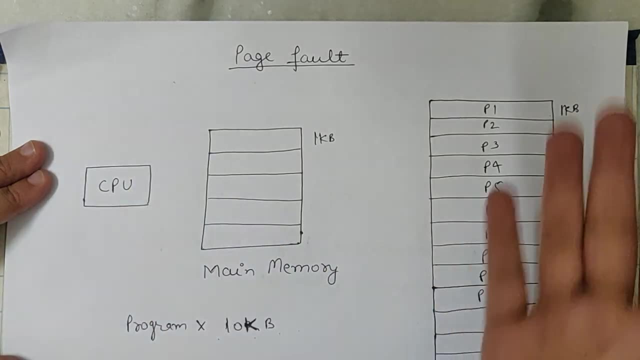 P4, P5, P10 and P11.. So initially these are pages, and each of this page is of size 1 KB. Okay, so it resides in the secondary memory. Now CPU wants to execute this program. Okay. 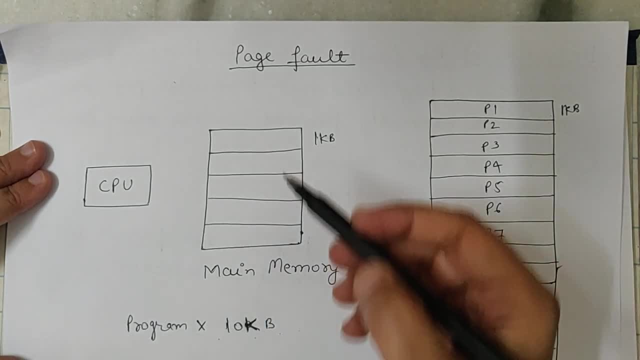 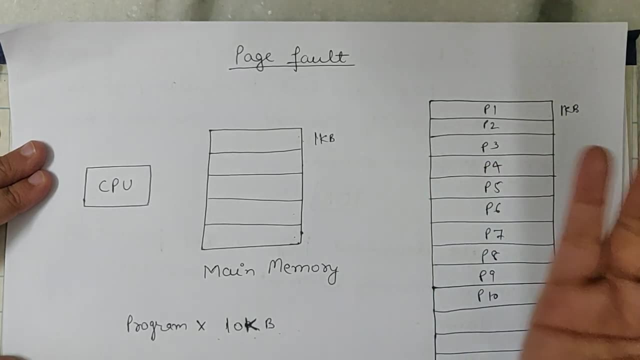 and we will load this program in main memory. but main memory is of size 1 KB plus 1 KB 1, 2, 3, 4, 5, 5 KB ka hi size hai. So initially 5 pages resides in main memory, say suppose. 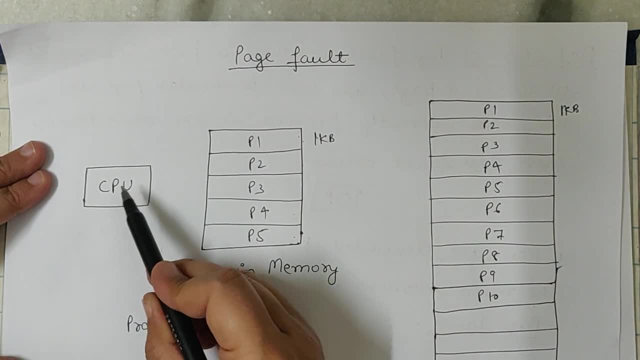 1,, 2,, 3, 4 and P5 resides in main memory. CPU quickly picks up: P1 page executed, P2 page executed, P3 page executed, P4 page executed and P5 page executed. Okay, now CPU demanded: 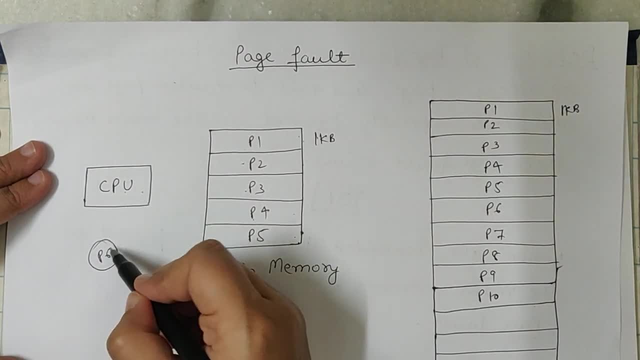 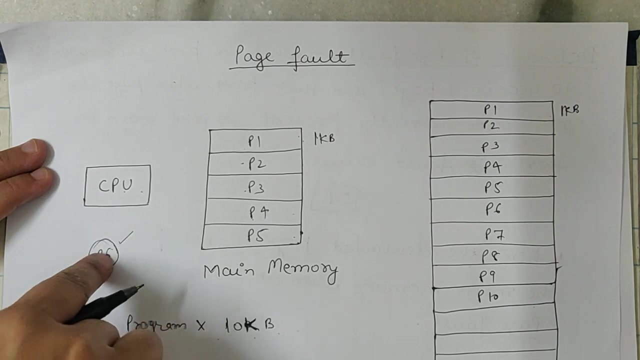 page number 6.. Okay, CPU wants to execute page number 6.. Okay, so now page number 6 is not present in main memory. This is known as page fault. When CPU demanded a particular page and that particular page does not present in the main memory, then that is known as page fault. Okay, jab bhi CPU. 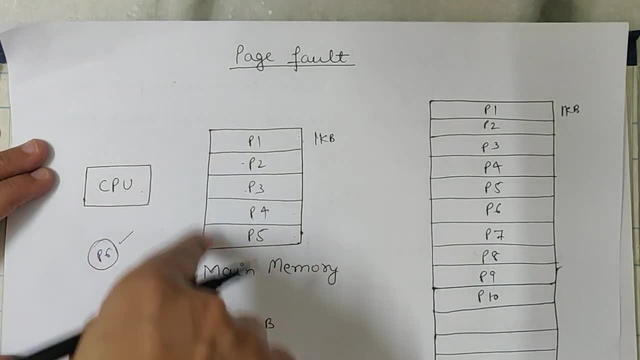 ko koi page execute karna hai, woh main memory mein page ko search karega, Agar woh page usko main memory mein nahi milta. ussi concept ko hum bolte hai: page fault, hogya Thik hai. 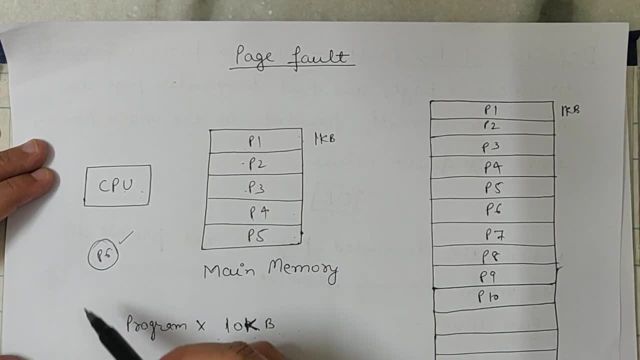 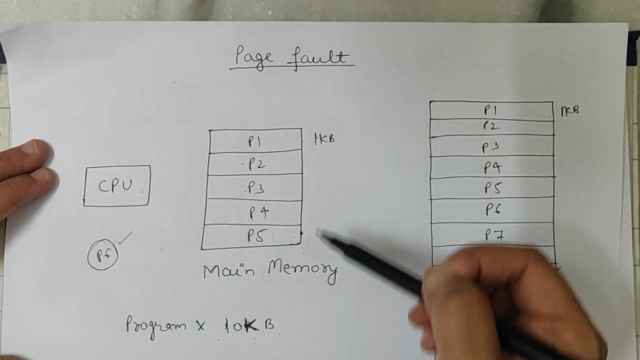 aur agar page mil gaya to page hit. otherwise miss Matlab page fault, Thik hai CPU. jab bhi kisi page ki demand karega, then it will search that particular page in the main memory. and if that page does not exist in the main memory, 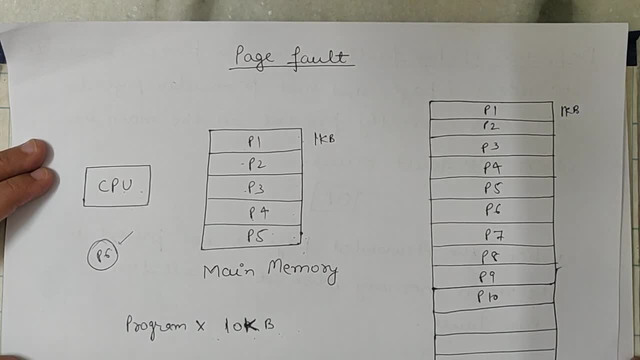 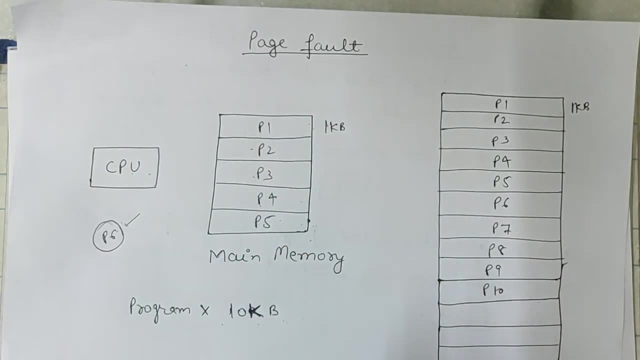 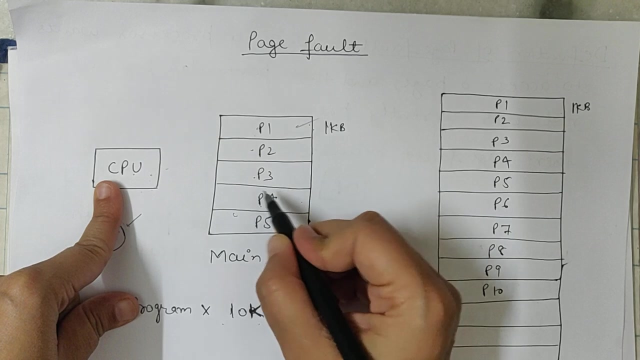 then page fault is there. Okay, so this is the whole concept of page fault, Ki humne page pages main memory mein reside kar diye. Jab tak to CPU ko pages mil rahe, the tab tak to hit ho raha, tha page hit. Matlab P1 usko mil raha, tha P2 mil raha, tha P3 mil raha. 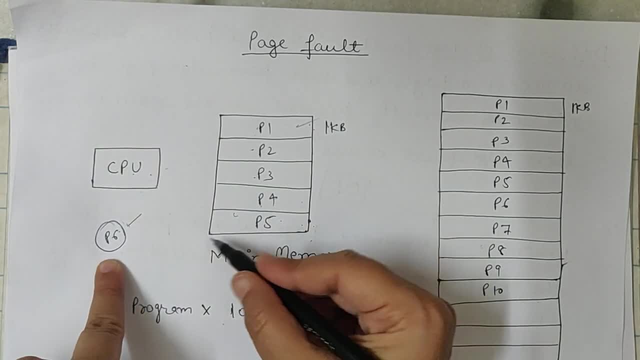 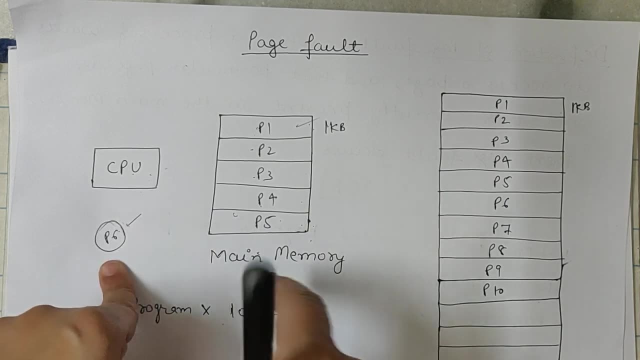 tha, and so on. Jaise hi usne P6 ki demand kari. P6 page usko main memory mein nahi mila To kya hua page fault tucker hogya Thik hai. This is the whole concept of page fault. Let's. 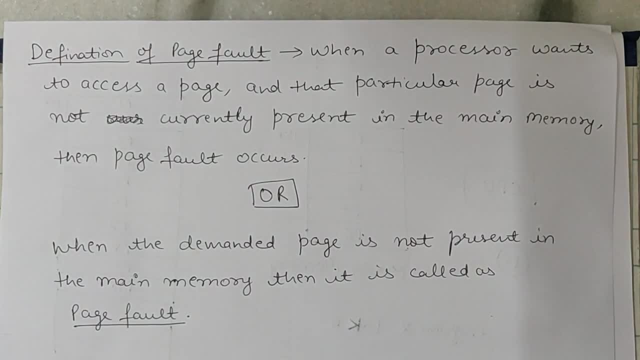 take the go through this definition. formal definition: When a processor wants to access, processor is nothing but a CPU. When a processor wants to access a page and that particular page is not current key Presently present in the main memory, then page fault occurs And ye definition mein. 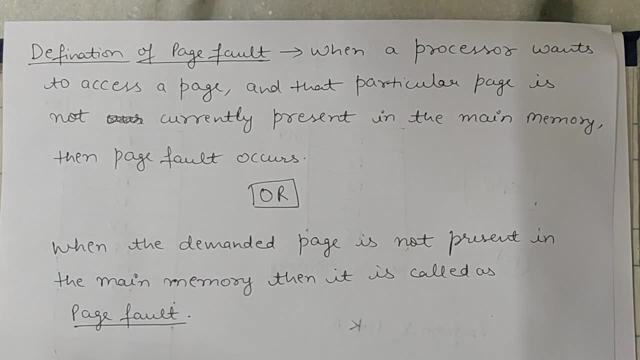 hum bol sakte hai. when the demanded page is not present in the main memory, then it is called as page fault. So if you want, you can take a screenshot of this Now, after page fault. okay, when page fault occurs Now, CPU wants to execute this page P6,, but 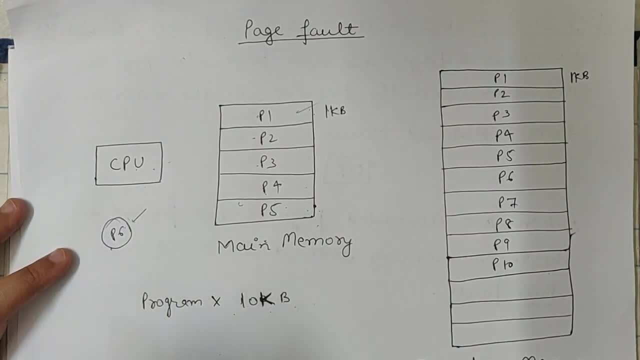 page fault hogya to hum aise thodi baith jayenge. We want to recover that page. na, we want that P6 page to be present in the main memory. So what we'll do is operating system. kya karta hai jab page fault nahi hota to hume page? 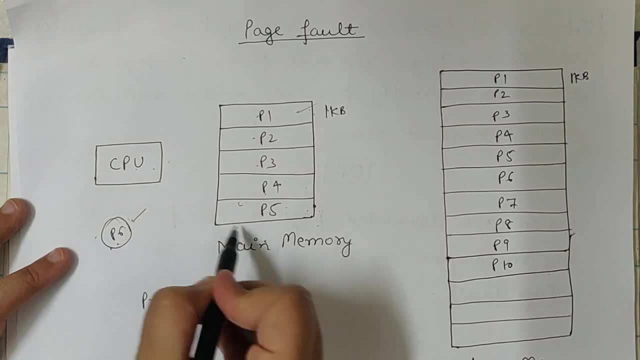 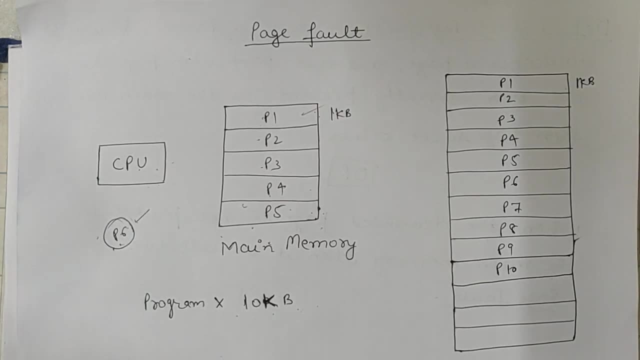 fault ko handle bhi to karna. padega Handle karna, matla P6 ko main memory mein lana padega, taaki page fault na ho. To uske liye hum kya karenge? there are few steps to handle the. 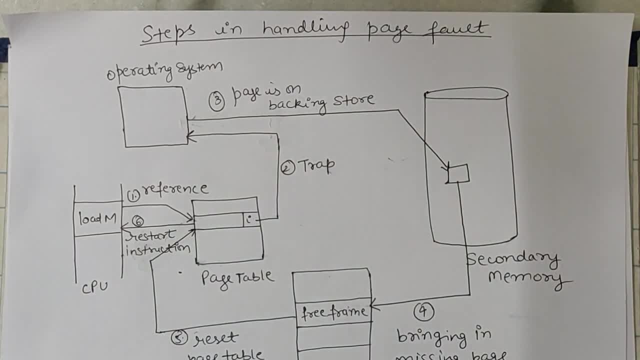 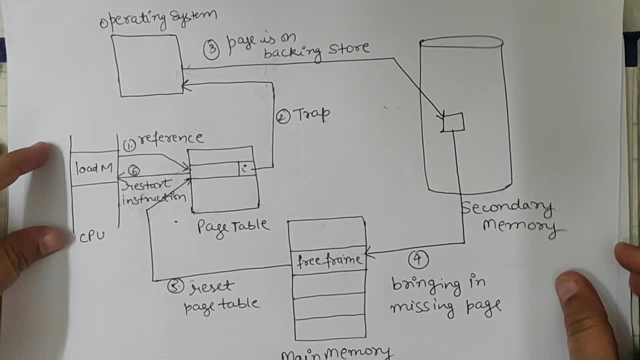 page fault. Let's see the steps. Yes, so these are the steps in handling the page fault. Ye dekhne mein apko thoda complicated lag raha hoga, but it's very simple. So let's go through this diagram. 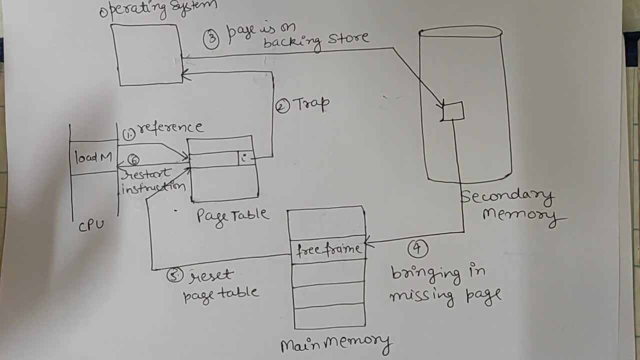 So let's go through this diagram. Yes, so these are the steps in handling the page fault. Ye dekhne mein apko thoda complicated lag raha hoga. Hellah is diagram mein, maine numbers likkhe mein. 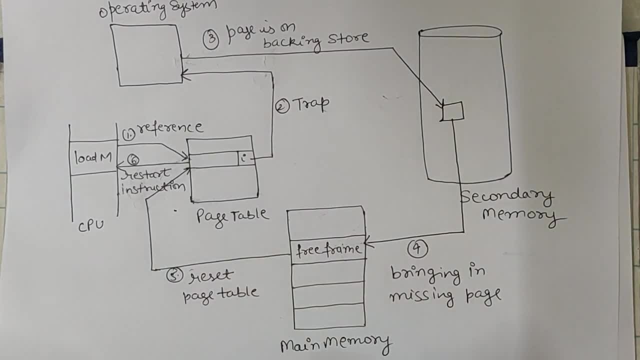 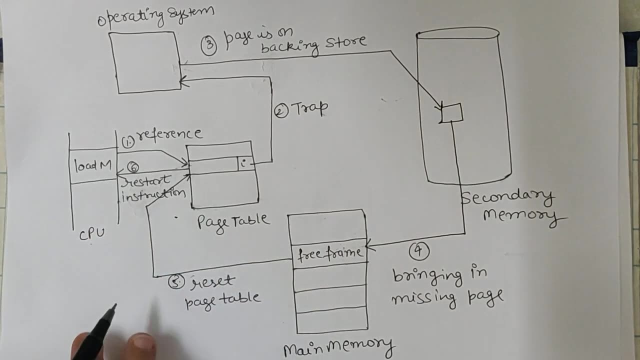 Ok, one, two, three and so on, Tikhe to ye sare steps hai. Abi, kya hota hai ye hai CPU. CPU want to load page number M. say suppose Tikhe ek page number M hai. CPU wants to load that page. 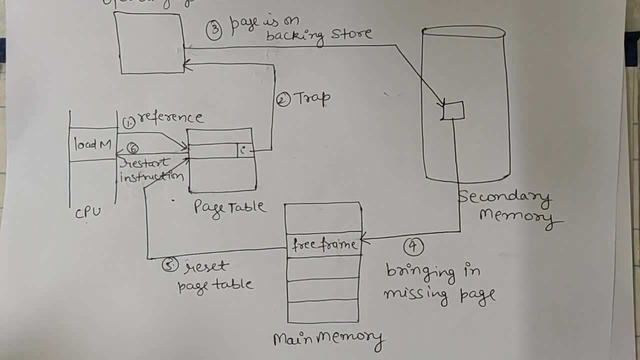 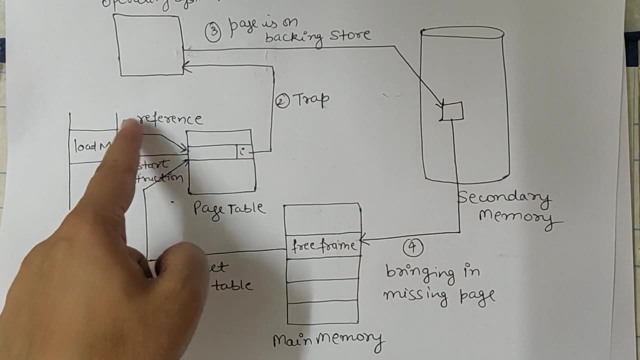 Wo gaya ye page table hai Ab har page ki entry hoti hoteенд page table mein Ye hamne dekha ta Address translation mein Page number 1, sorry. step number one is Reference matlab load M. Load M ka matlab hai ek page control. 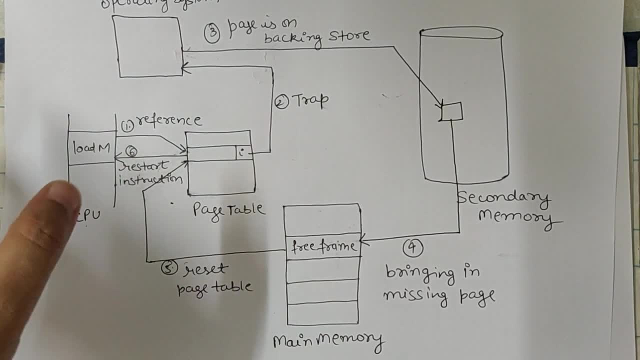 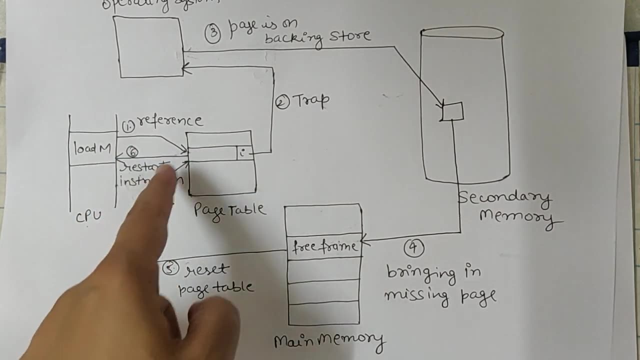 enti, in this case number 2.. No, no, no. so in that case we want to load that page. we have taken a page whose name is M. CPU wants to execute that M page. CPU has referred to the page table. its entry is there. 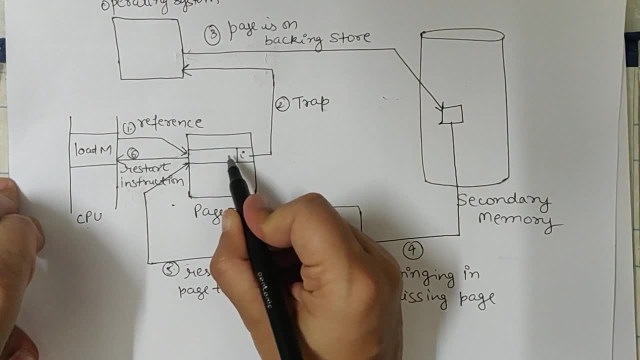 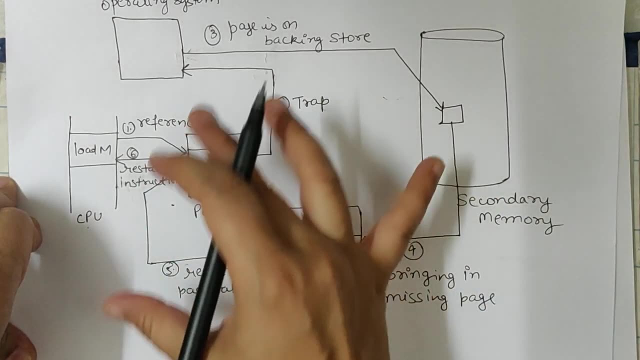 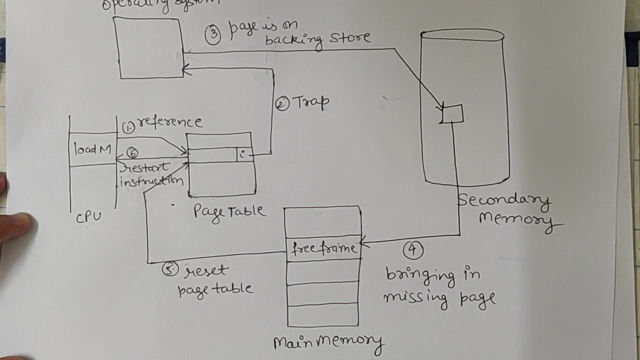 what is it checking in the page table? that in which frame number, M page number, will reside in the main memory. it wants to check that in the main memory. as we have seen in the page table, every page number is known in the main memory. in the same way, when CPU wants to execute, 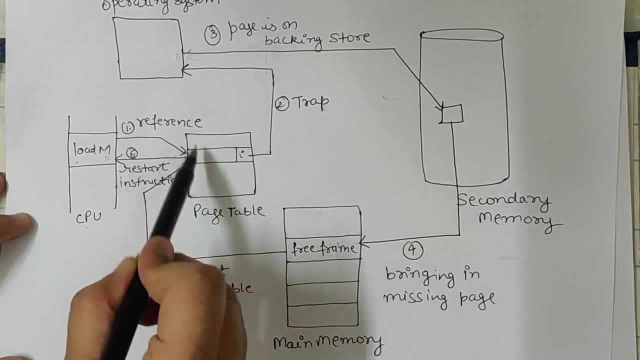 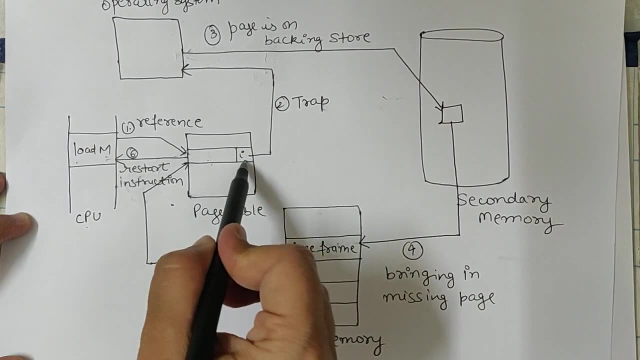 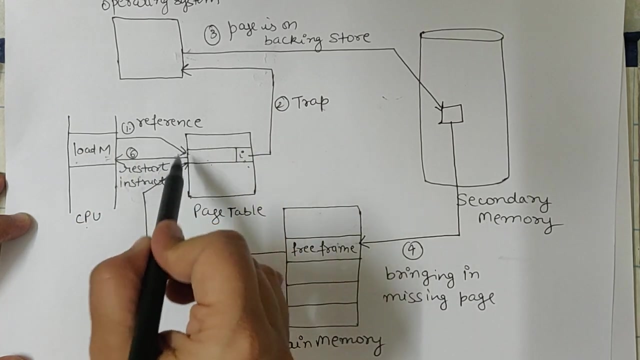 the page number M. it will check the entry in the page table in which frame number that M page number is. we are assuming that it is not there. I denotes invalid. this M page is not residing in the page table. this is an invalid entry. I means invalid bit. 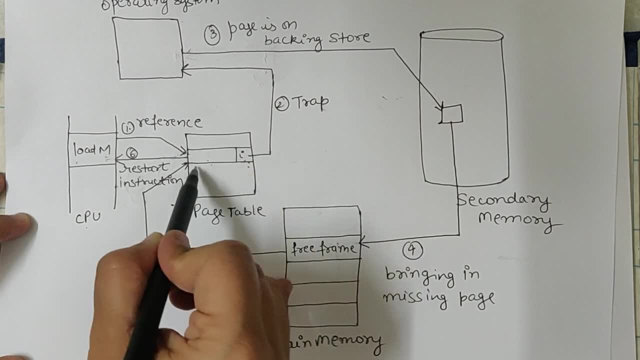 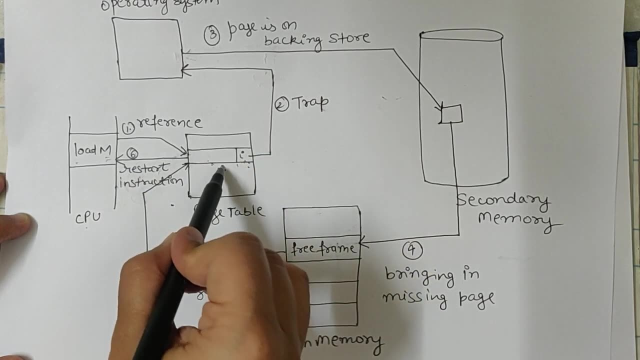 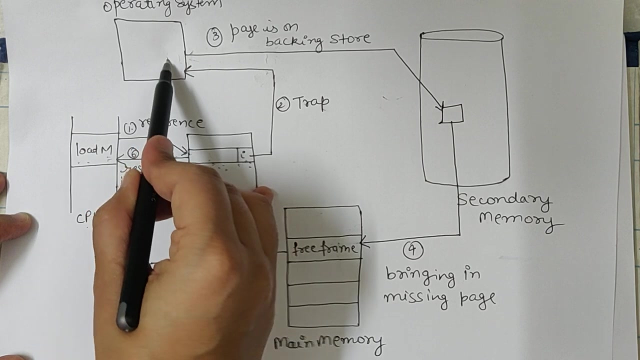 M page number M is not in the main memory. it is not in any frame. M page number. M page table tells that you are searching an invalid page. now, if it is not there, then the second is a trap. it has sent an error to the operating system. 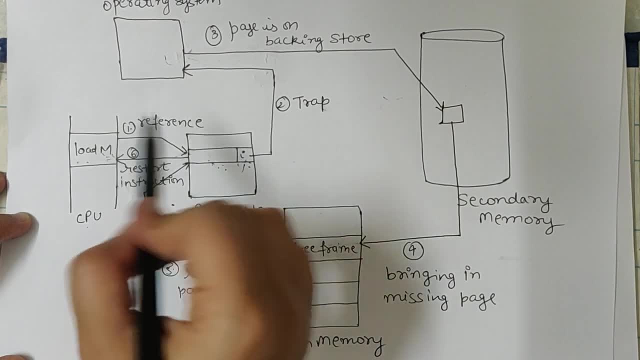 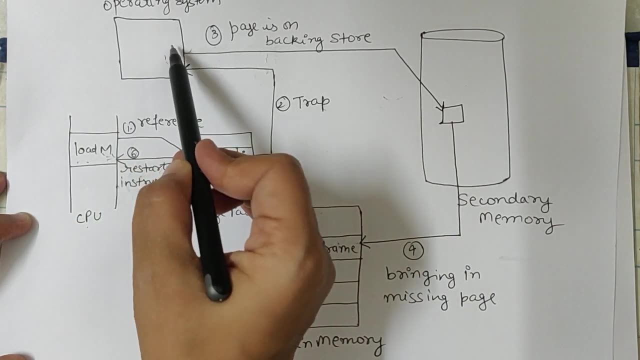 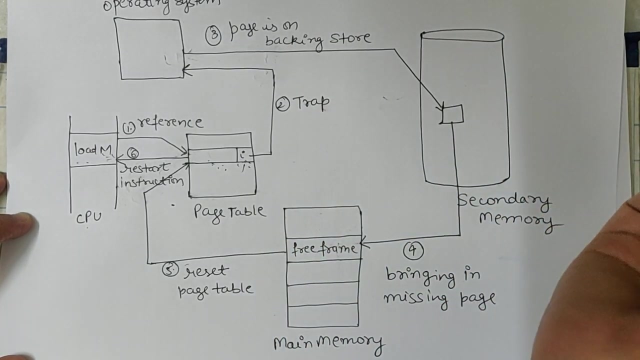 we are recovering, our page is not there. M page number is not there. now the operating system is a process control block in which all the pages are entered, whether it is present in the secondary memory or not. so the operating system will go to the PCB and check whether the page number M is present in the secondary memory. 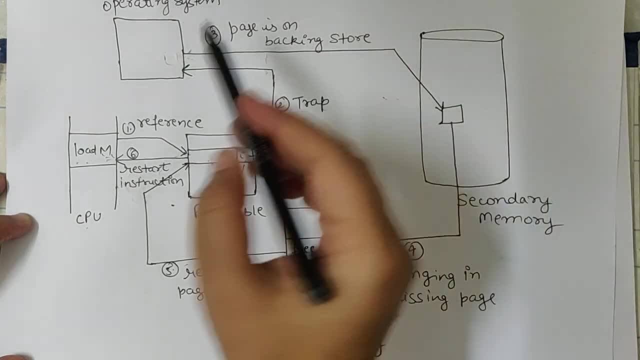 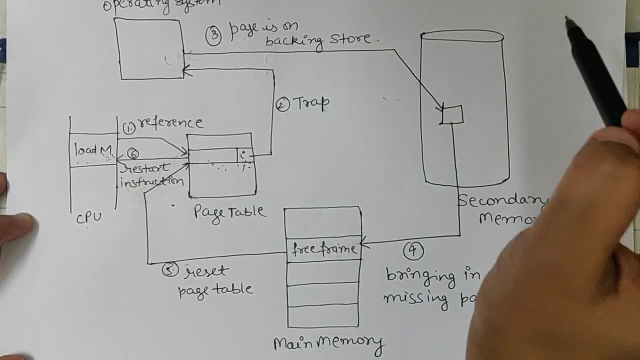 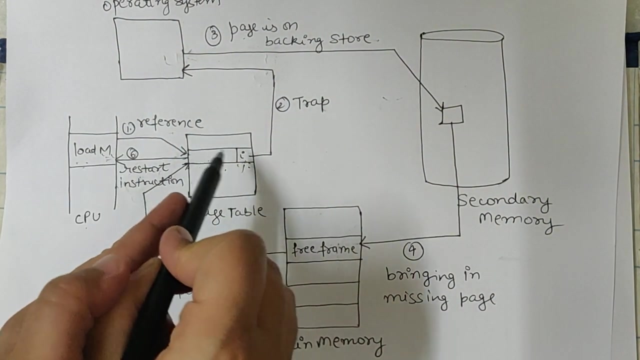 if it is there then it will tell. page is on backing store. backing store means secondary memory. it is in the hard disk. CPU has sent the requirement of M page M. page number M was searched in the page table. that page number M was not in the page table. 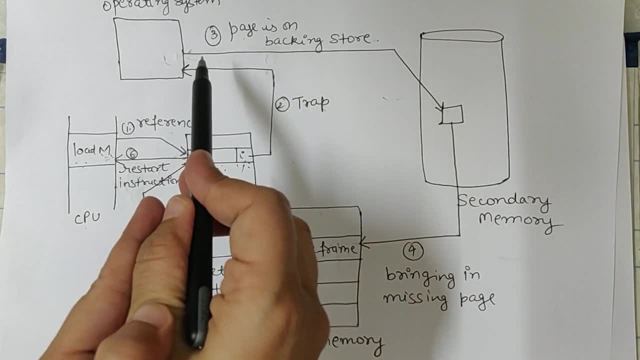 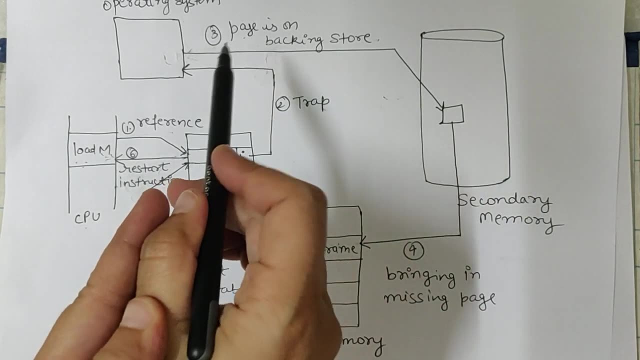 so it has sent an error to the operating system. operating system has found out whether that particular page number M is residing in the secondary memory or not. as soon as it is residing, it has given a signal. page is on backing store now this particular page number M.